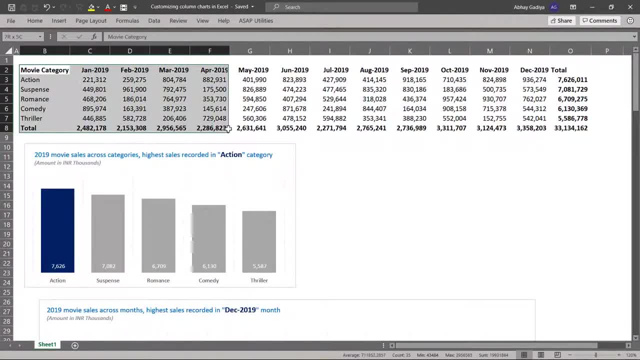 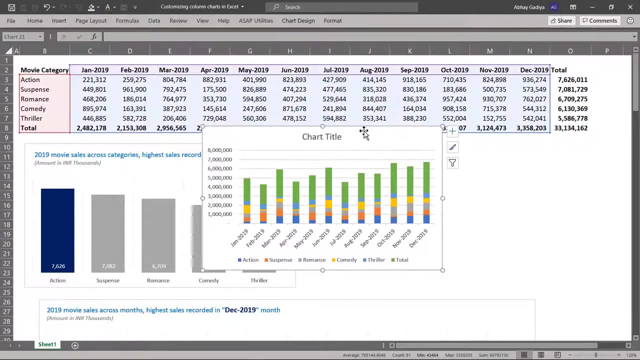 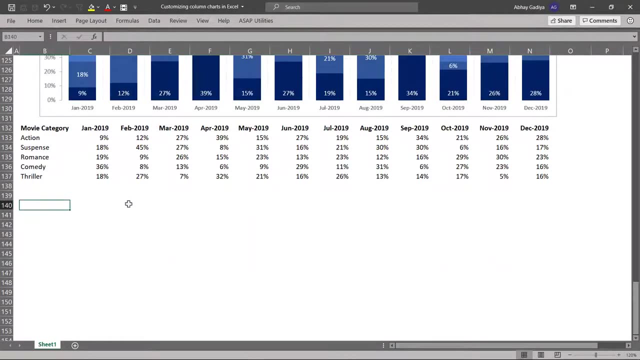 So let us go and select the total rows also for that given month. Let us select inside Insert. Then let us select stack column. This time we are selecting this Control X, So let us move that to bottom. Let us control V. 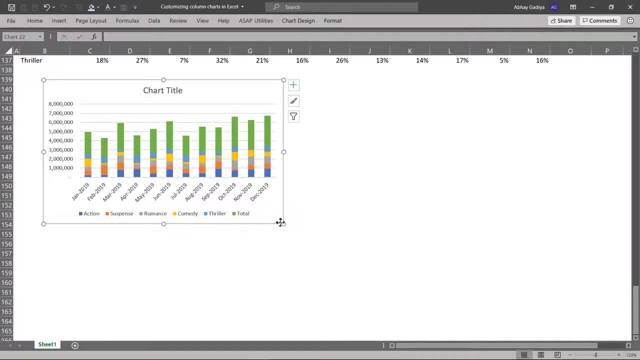 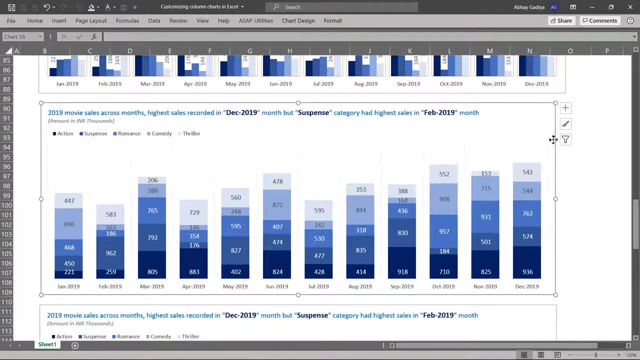 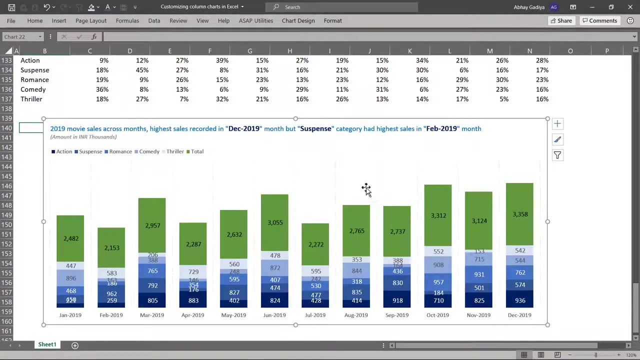 Now let us change this column width and height by dragging the borders. Let us copy our formatting from our previous chart by selecting this chart, Control C, Then Alt E, S. Let us click formats. Our formatting is getting applied. Let us go to chart design. 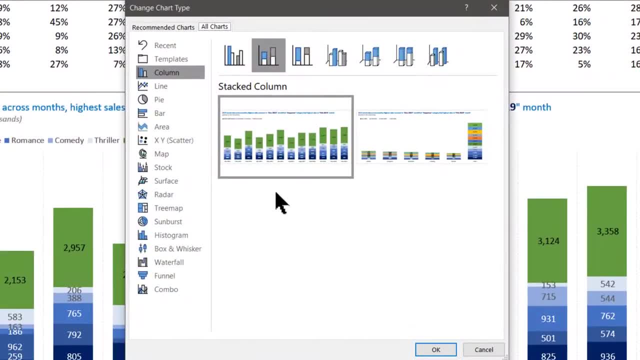 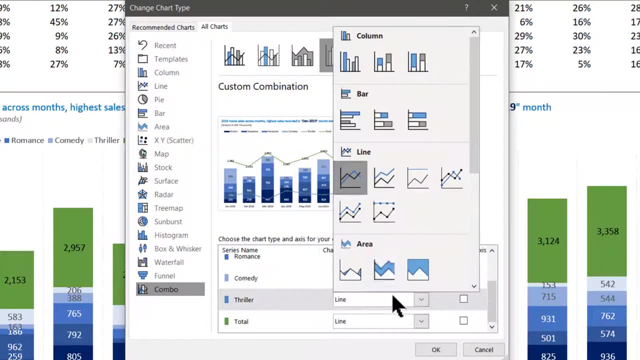 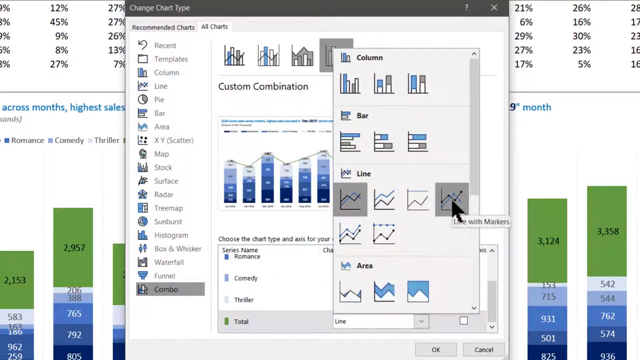 And this time we'll be selecting combo charts. All other charts should be stacked column, So everything is stacked column. Even Thriller also will be a stack column And this will be a line chart with markers. So line chart with markers we will have to display. 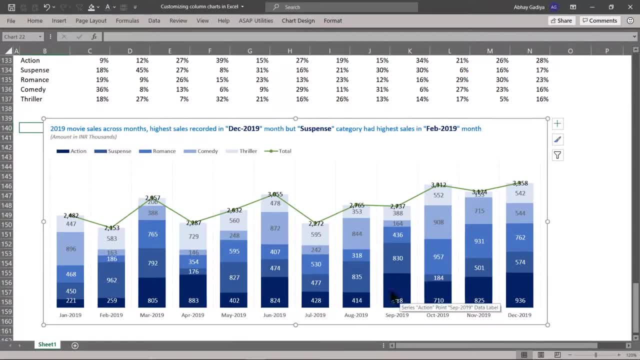 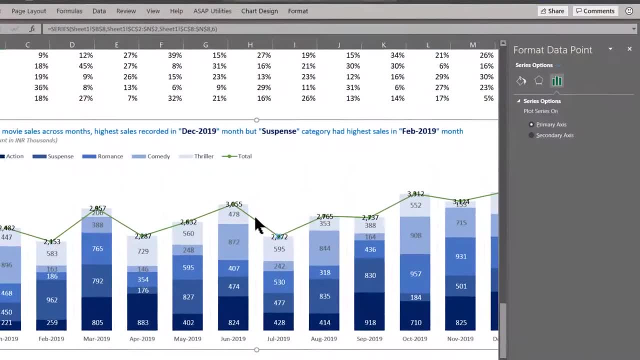 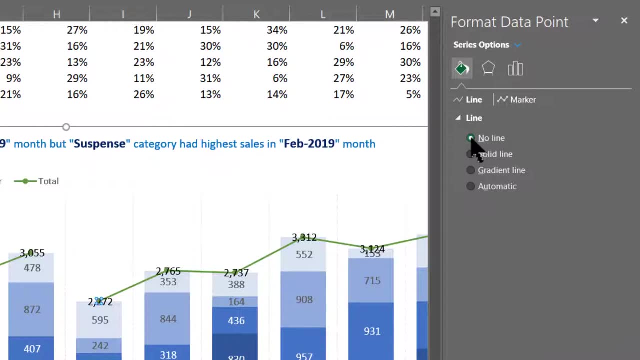 So let us click OK and it gets displayed something like this: Let us select this total one, And now let us print it, And now let us press control one. So now, once this window is opened up, So let us go to solid line and we will select no lines. 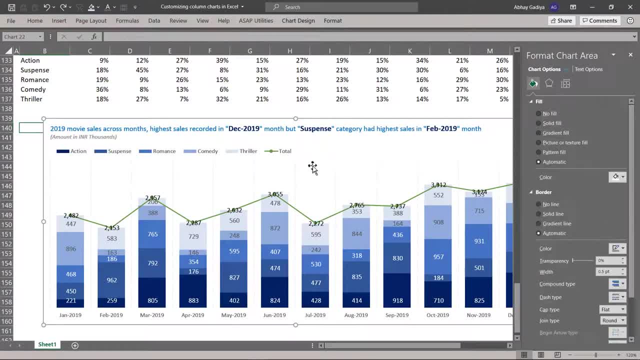 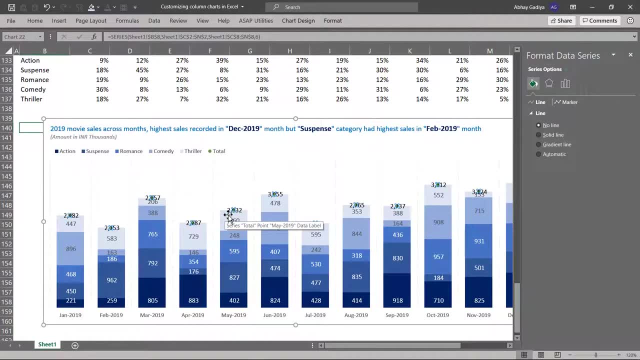 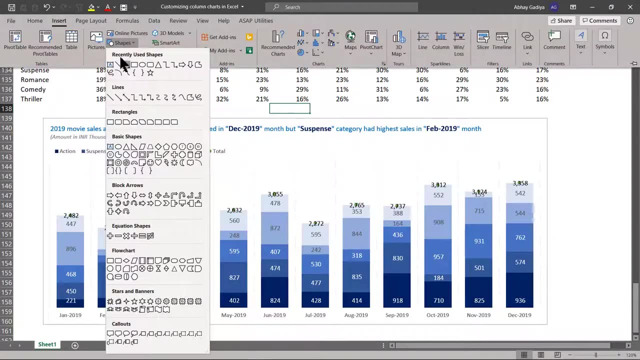 So uncheck this. So, since only a single line was selected, So let us select entire thing and then select no lines. And now only our markers is being selected. So let us change that marker by inserting our shape. So let us go to insert shapes. 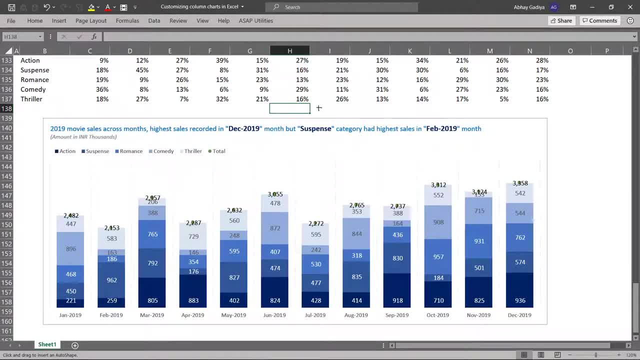 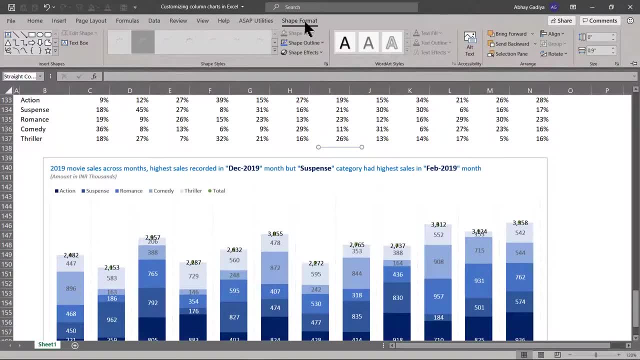 This will be a horizontal line. So let us press shift and then draw a horizontal line, Just like we have done it for other charts. Let us go to shape. Let us change the color to this orange one, Let us change the weight to this one. 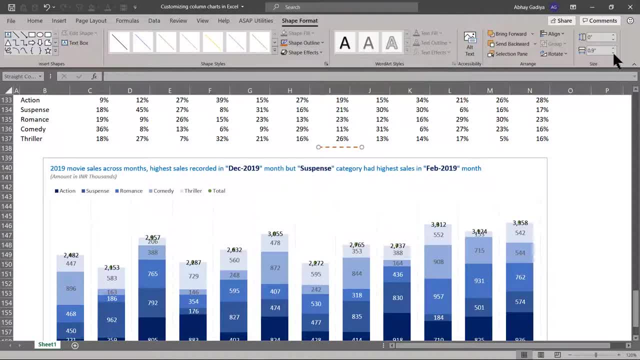 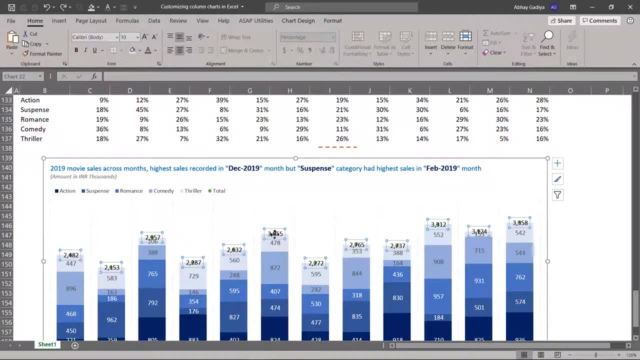 Let us change the dash type to dashes And let us copy this. Let us select this control C, And now we will be selecting this markers circle, And let us press control V, So this will get replaced over here, And now we will be displaying our data labels, also for this total one. 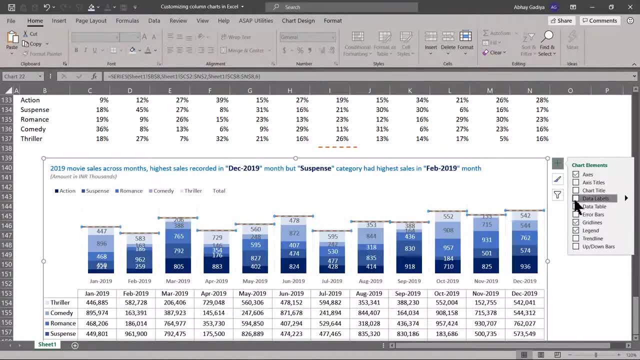 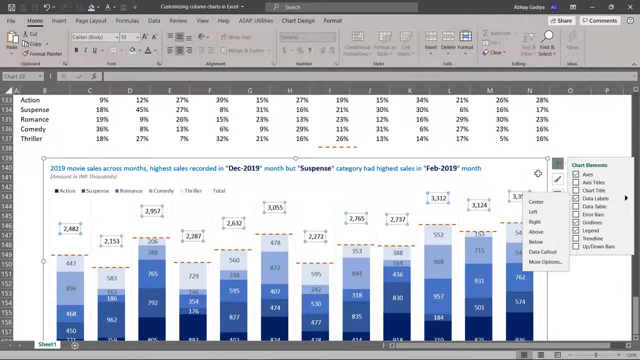 So let us select this. Go to data labels. This will be data labels at the above this one. So once you have selected that, let us change the color for font, And this will get exactly displayed something like this. So now we will have to drag this dash.